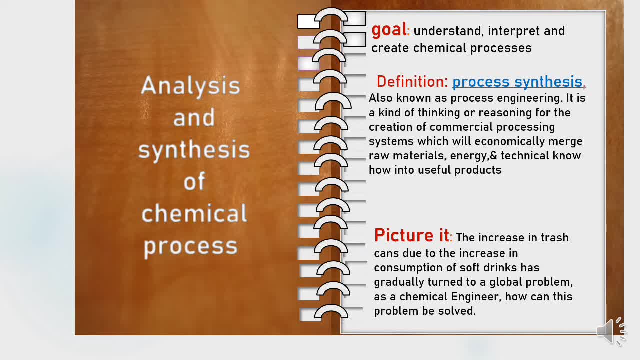 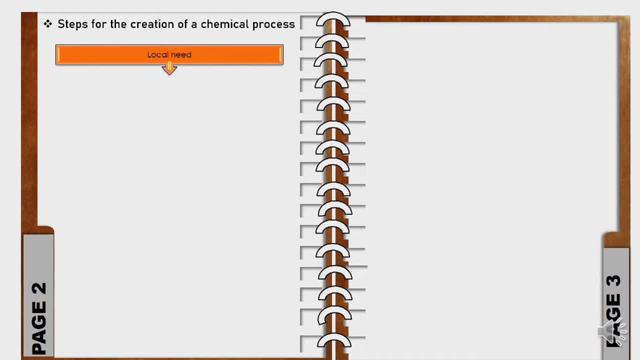 then can this problem be solved as a chemical engineer. So let's see So steps for the creation of a chemical process. We have the local need. identify a local need, which we just did. We just identified a local need in which the local need is how we can. 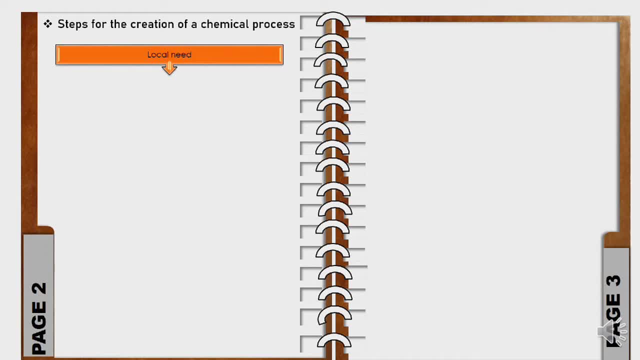 actually handle the increase in trash cans due to the consumption- high consumption- of what soft drinks So, ranging from Coca-Cola products, ATC. how do we handle this so as not to pollute the environment and later the environment with biodegradable, non-biodegradable? 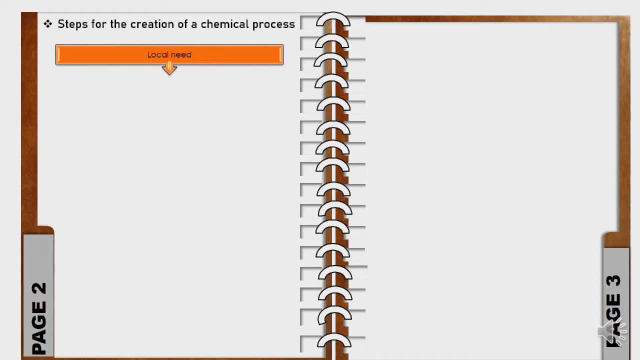 materials. So how do we handle that? So, identify a local need first. Problem with definition. Define the problem, Convert the problem to an engineering problem. Back then in high school we treated word problem, in which we transformed the word problem to a mathematical problem. So here, 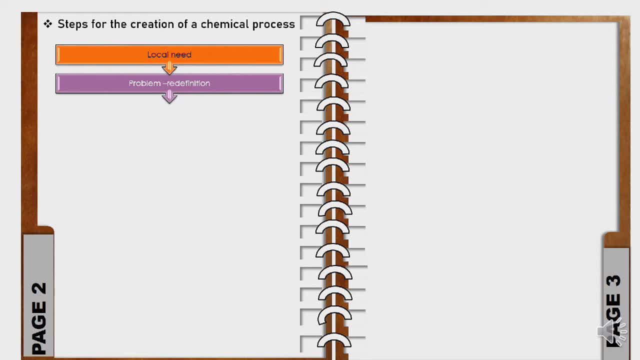 what are we doing? We are trying to convert a local need into an engineering problem for further studies. And how do we do this? We can only do this by gathering information, mass information on the problem. The next step will have the process configurations Generate different possible ways in which. 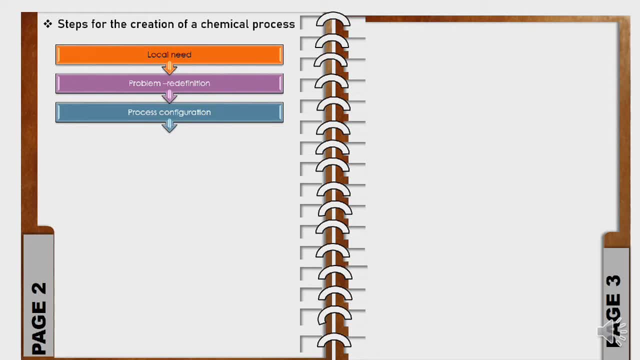 we can solve this problem: Different possible ways of handling these trash cans, Different possible ways of either recycling them or how we can handle them so that they don't litter the environment, so they don't pollute the environment. So is the process feasible? 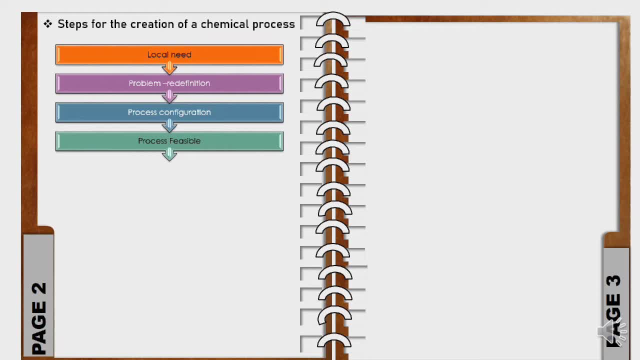 These different ways are generated. Is this something that is possible? Is this something that can be done? If no, we'll go back to the problem definition and try to reconfigure the problem again to suit what we need. If yes, we'll go ahead and then design the process So, when we are 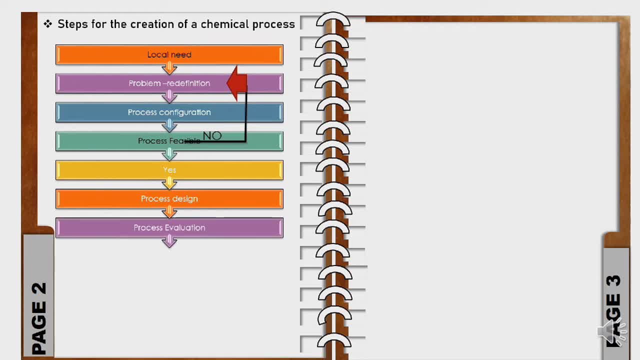 done with the design of the process. we will now evaluate the process. What is the cost? What do we need to put these things in place? What is the machine that we need? Construction of every other thing. What is the cost of putting these materials in place? that will? 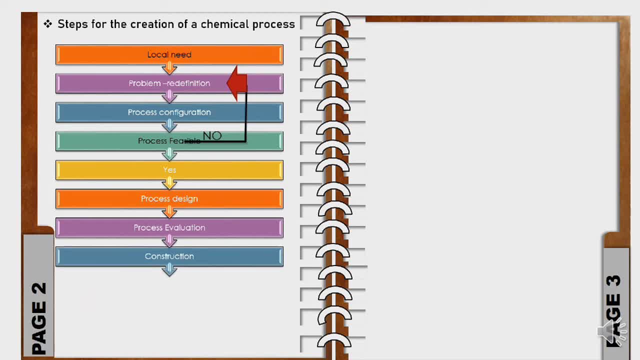 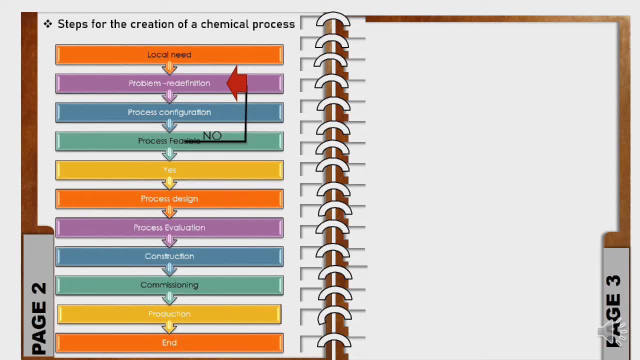 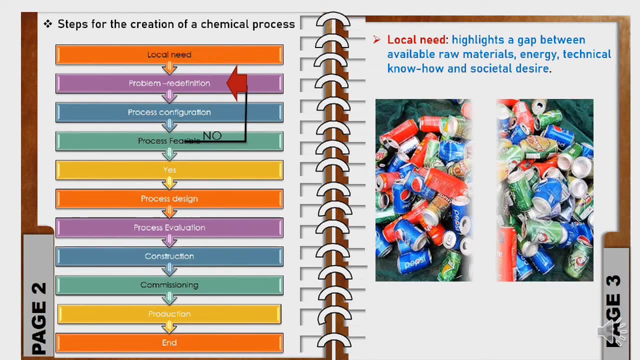 that's the end of the whole process. So these are basically the steps for the creation of a chemical process. Let's look at this, The location of it. That's what I just said. This location that I can handle is becoming too much in the environment. So, as chemical engineers, what can you do? 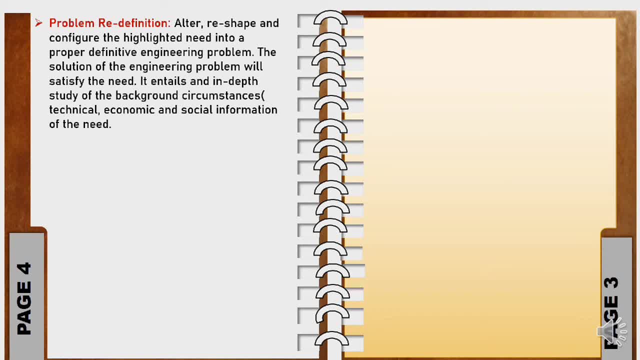 okay, so we talked about problem redefinition. so we've talked about this. you reshape, you configure the highlighted name into a proper is there for us so you can refer to that. i've explained that in the former slide. so the third process. so this is just a guide on how you can. 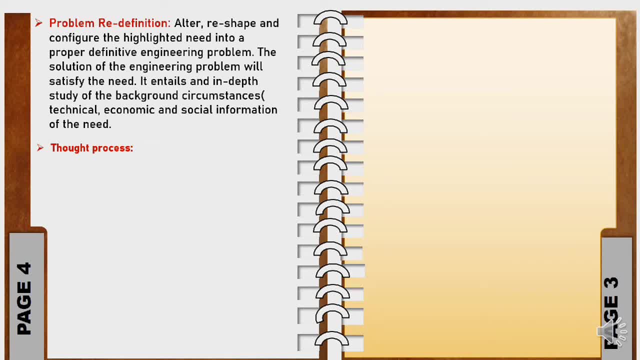 actually configure a problem to an engineering problem. so, just a step, just like in high school, have the steps. you can do that. if you also did your linear programming, you also have the linear programming, which will not convert to an engineering problem. okay, so that was the same. 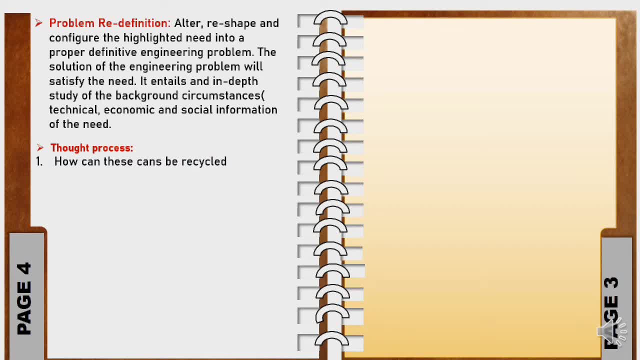 thing. the third process: how can these scans be recycled? can we recycle them? so how can we do that? what is the quantity needed? what quantity can we gather so as to recycle them? so what is what is needed? how can we reduce the quantity that is disposed? how can we do that? 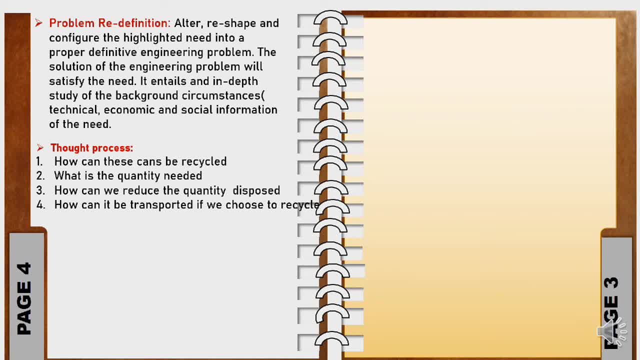 how can it be transported? if we choose to recycle? how do we not move the cans? after gathering the cans, how do we not move it? these are things we consider, then. what kind of machine can recycle this? so this forms? these are the thoughts process that will help us convert this local need to an engineering. 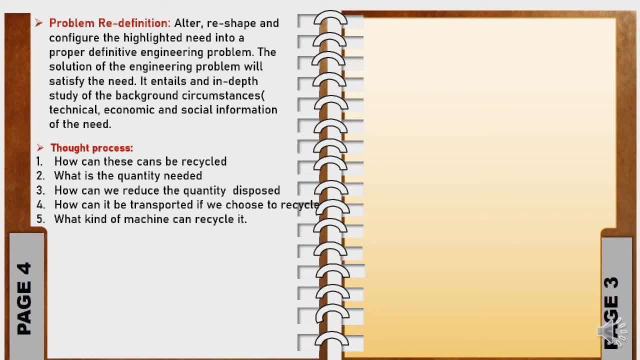 problem. so that's it, the five basic step, or the thinkings or the thoughts you can put in place to convert a particular need to an engineering problem, and then the process, configurations, different possible ways we can solve this problem. that will highlight it, the solution to this. 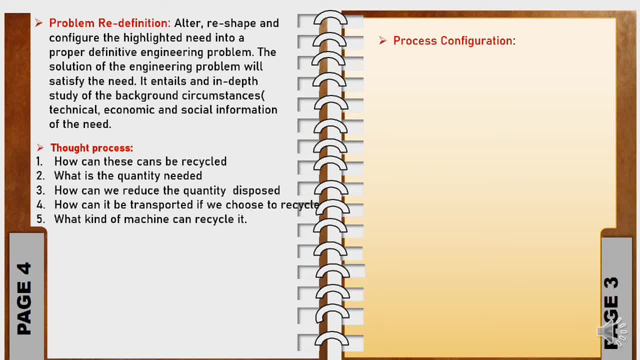 the solution that we're going to amass here will not help us to solve that. look at it. so let's see: synthesis of feasible, generate a lot of them, but will not select the best, the best, which now forms the solution to the problem. so that's what it means to say: synthesis of feasible and plausible. 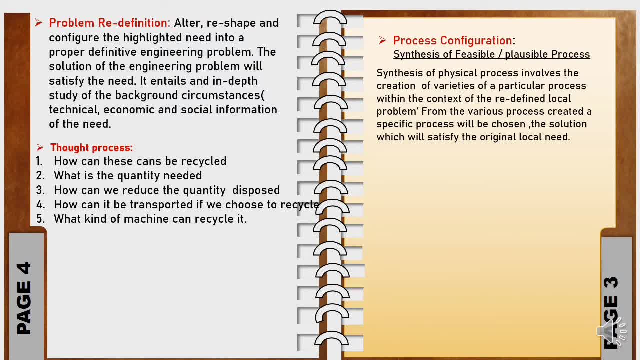 process. so that's what we mean: generate various possible ways. you can solve this problem different ways. you can solve them different ways. you can recycle, discount different ways. you can choose to um gather them different ways. you can choose to transport them- different kinds of machine that can. 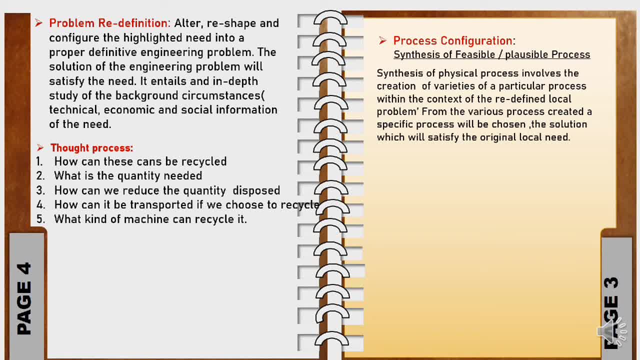 do this work? then, after these different processes, the goal is not to select the best, select the best out of it. okay, so that's how, what we'll do. so how do we now create this plausible alternative process? how do we do that? the same step: define the problem, convert to engineering problem: um data. 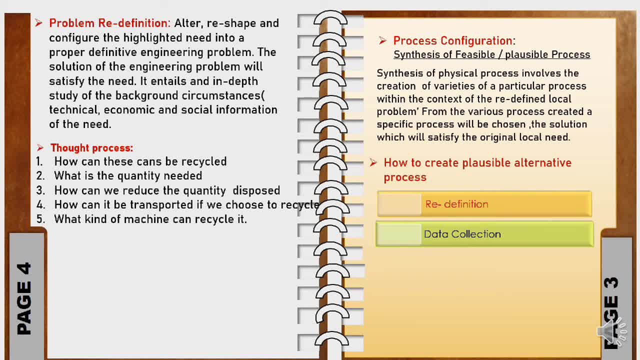 collection. collect, sorry, data collection. collect information, the pertinent information on this very problem. gather information as much as you can through books, through questionnaires, through other people that have done such work. gather as much information as possible. so when you've done that, you now generate the process configuration based on the information you obtained, the different ways. 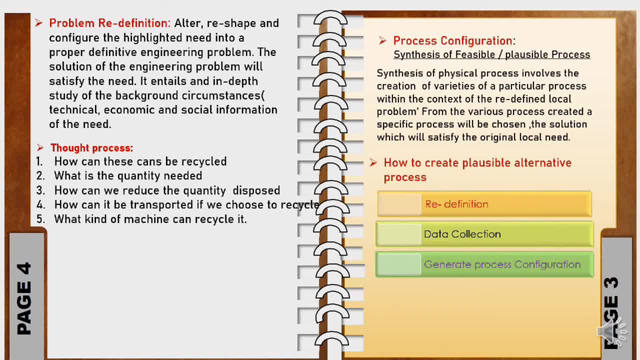 you can recycle from books, from resources that we need to do from there, which are in the process. so you now sell. access the process. so in the next slide, 100 different ways. what are the criterias? how do we assess the process? i'm not the one. that is best. you now select the optimal. 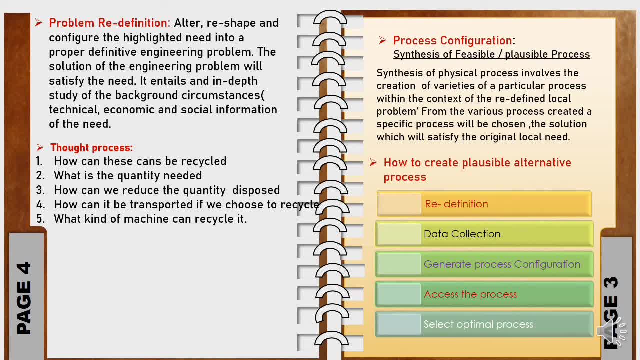 process. that's the last step in our process configuration. you now select the optimal process. as a chemical engineer, our goal, our aim, what we need to do is just to select the optimal process: optimization, either to reduce cost, you know, so as to reduce cost, or maximize profit. this is 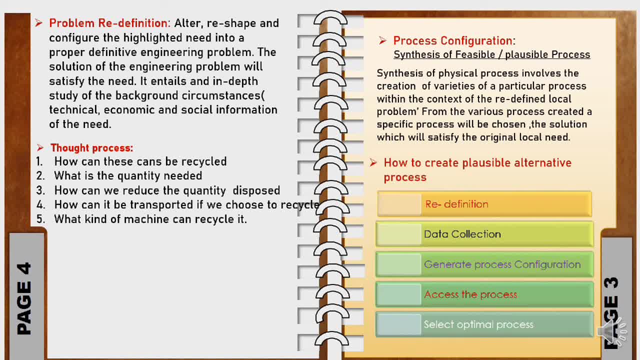 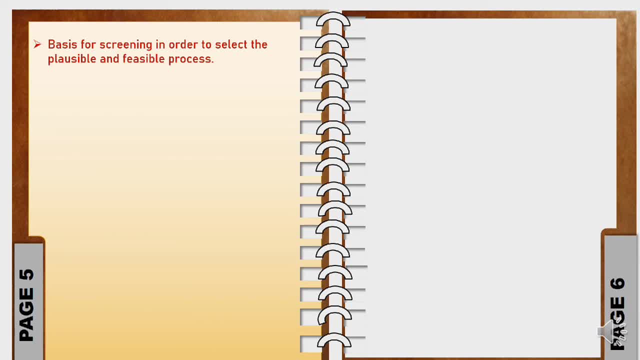 the two basic things that we'll do in engineering. optimization is very, very important. so what are the basis for screening? how do i know that the process is good? how do i know you want to select? so this will guide you. number one: logicality. is this something that follows logical reasoning? 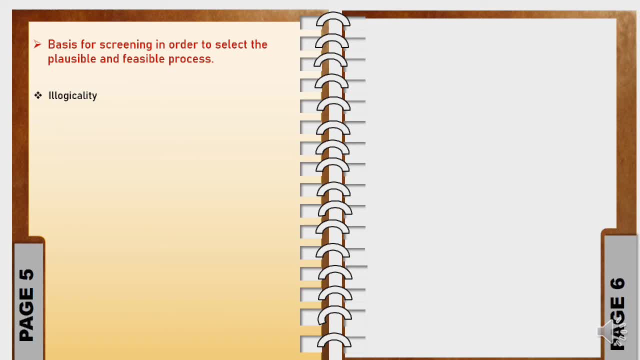 it should follow logical reasoning, it should obey scientific laws. so if a process or the way you want to recycle they can, the way you want to better these cans for recycling, if it doesn't follow a reasoning, if it doesn't obey scientific laws, that means you have to screen out such a process. 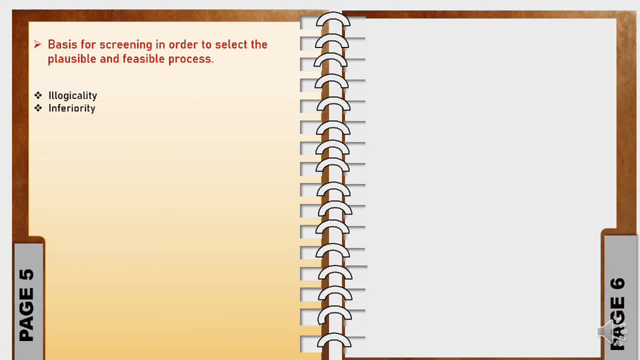 you talk about. if it is not an improvement to already existing technology, we have to live it out. it must be an improvement to what we used to know you are trying to improve, you're not going back. it should be something that is superior to what we need to work before. so that's one of the 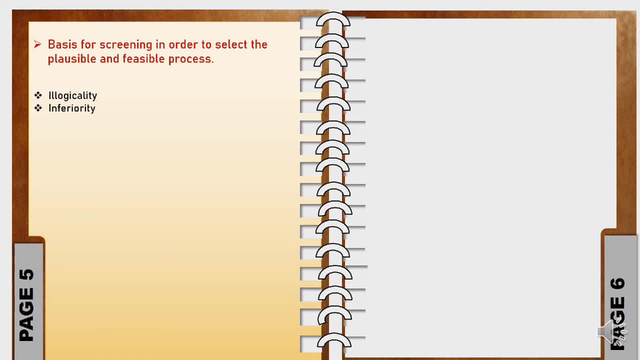 basis. if it is something that is inferior, then we are leaving it out, so it should be an improvement to radio system technology. next one: safety. no matter the amount of money, no matter the profit will come back from a particular uh process if it is not safe, to both depression and to the. 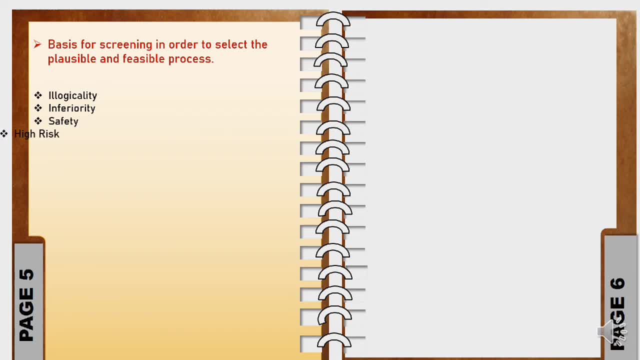 environment. we'll leave it out. so that's one of the basis for doing this. then the risk. you have to check the level of risk. if the risk is too high, it will screen out such process. for instance, different people or different ways: different person might bring out different ways with a. 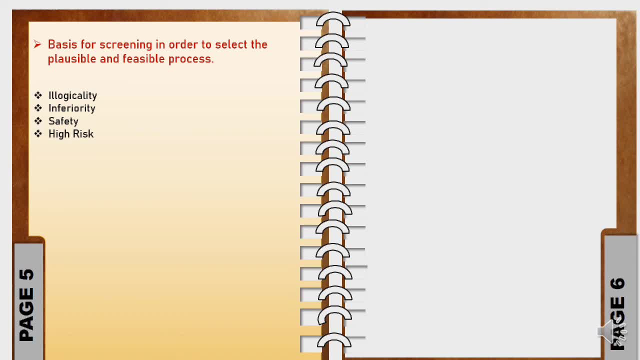 recycle discount. we have to weigh the risk. which one has the highest risk, so we'll not choose the one that the risk is minimal still optimization, so it's very important. so now, how do you obtain information? there are different ways you can obtain information. i've mentioned that academic area feeding, virus standard and practice. 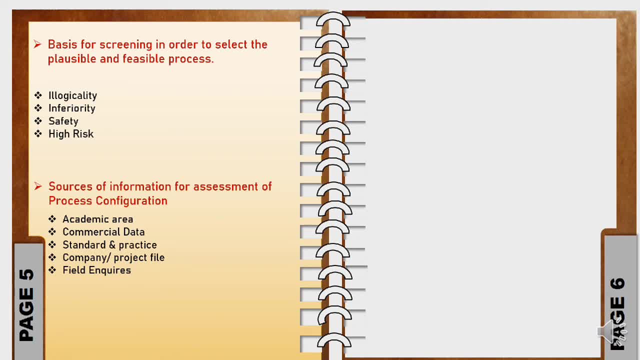 commercial data. these are different ways you can collect data that will not help us to generate our process and that will also help us to know whether to screen a process or to leave it. it is from the data you've collected that you will not know that this particular process is good. this particular process is safe enough, is an improvement already. 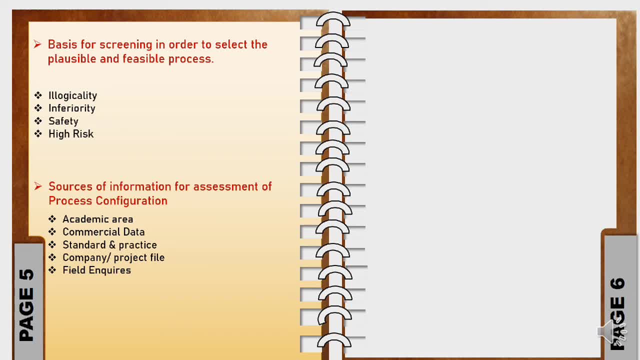 existing technology. it is when you study books you will not know that social and social process might not be good. okay, so that's the social information for assessment of process configuration. okay, and in the next class we'll handle the process design. so on that process design, we've. 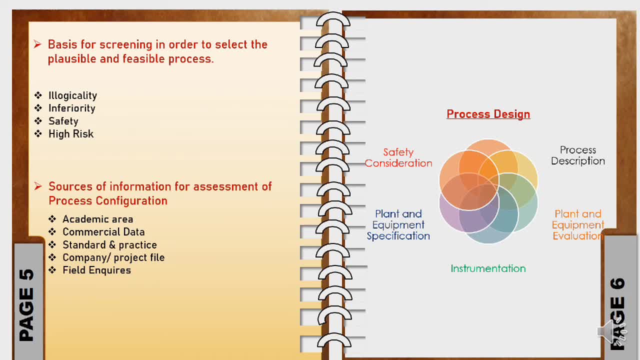 directed a good process. we've selected the best process. we'll now go ahead to design the process. we'll have the plant and equipment evaluation just as you can have you see here using the smart app. so that's all we have. so in the next class we'll dive into the process: design and basically.